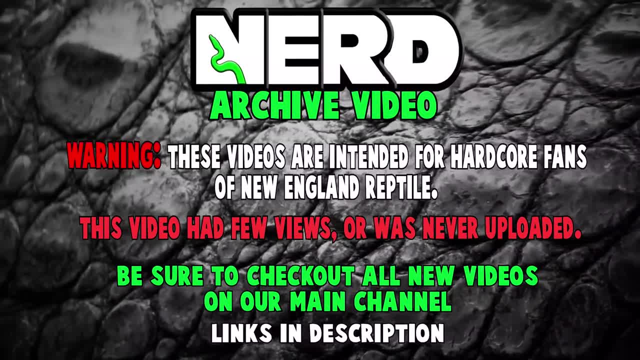 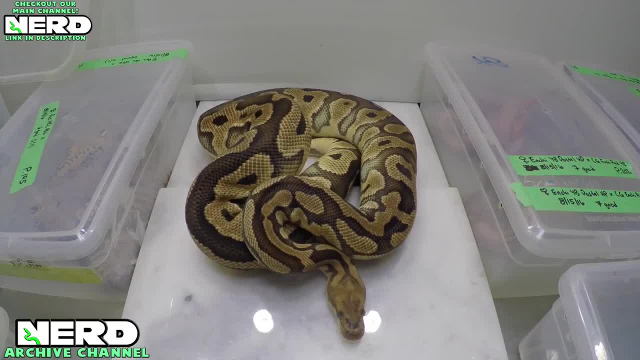 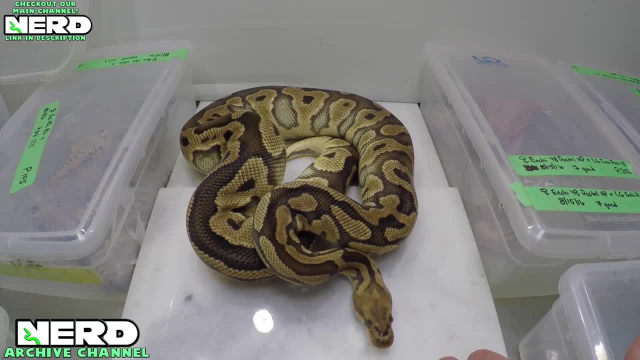 All right, I'm going to do a video on recessive genetics, And recessive genetics is very important when we're dealing with a python species that we're breeding captivity. So in this case we're going to use a clown, But another parallel would be albino caramel, albino ultramel. 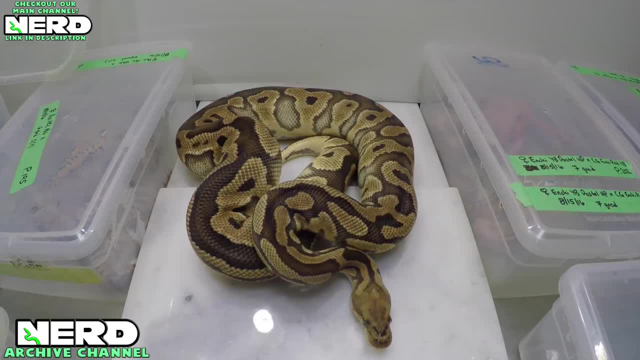 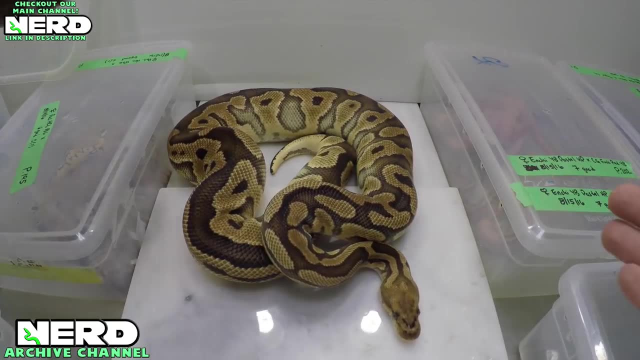 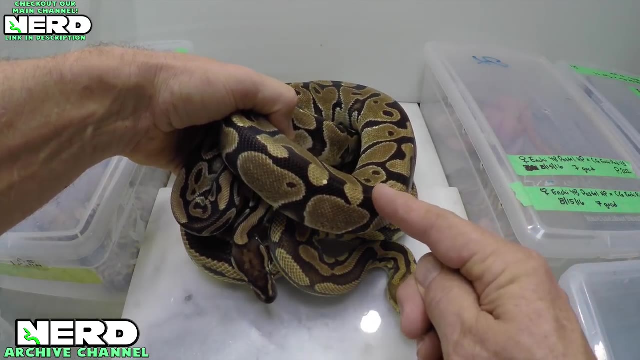 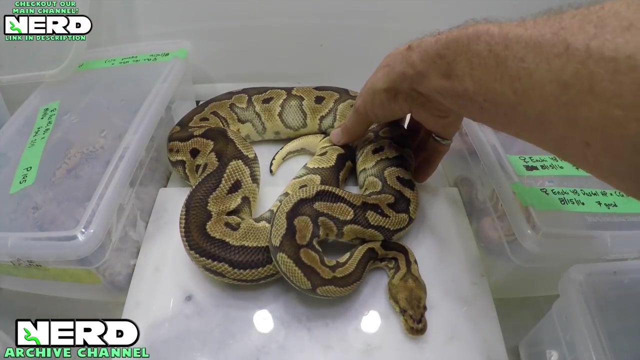 piebald. But let's go to clowns. Clown is a recessive gene which means when this snake is bred to the normal wild type, the wild type appearance is dominant to the look. So when I breed this snake to the recessive clown and I make eggs, 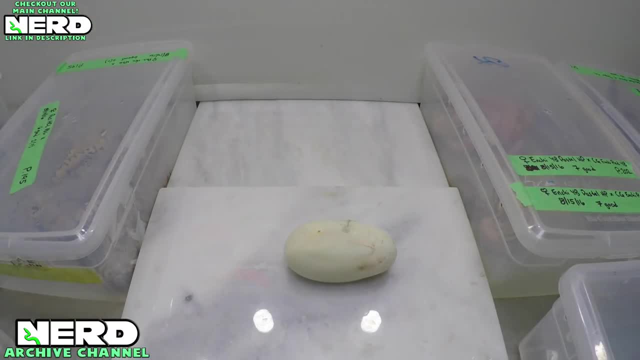 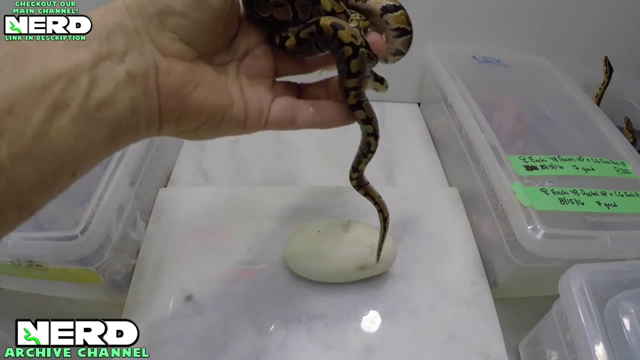 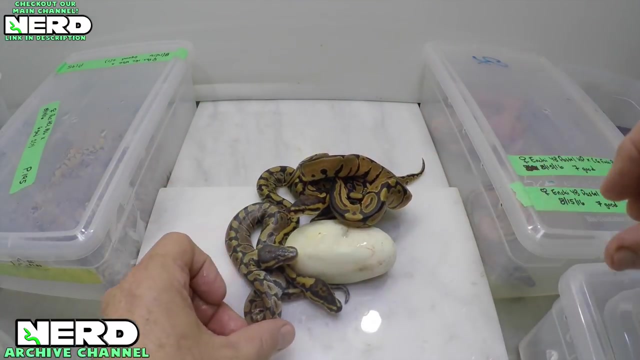 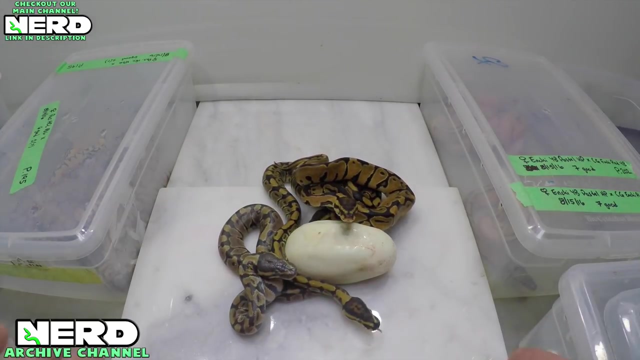 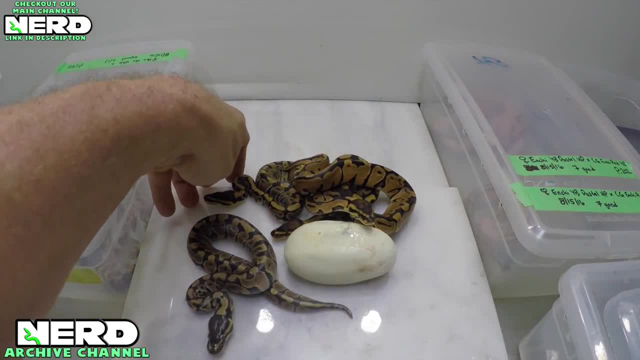 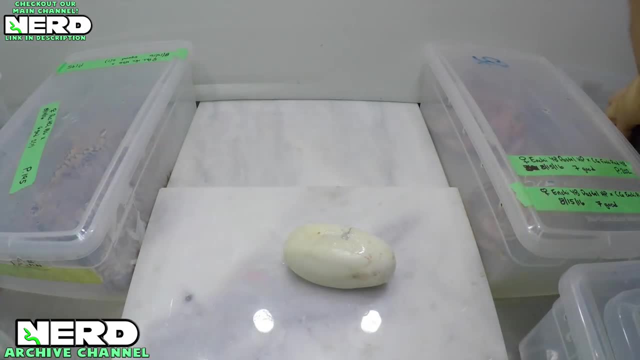 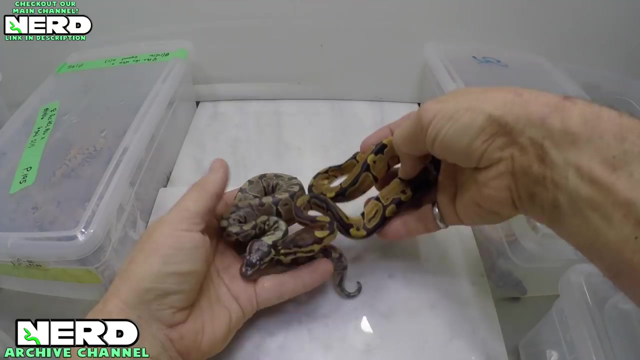 But the other parent contributed the wild gene which is dominant, So it basically masks the occurrence of the clown. So if I take those hets and I were to breed those together. so I took a normal-looking and a normal-looking, both het clowns. 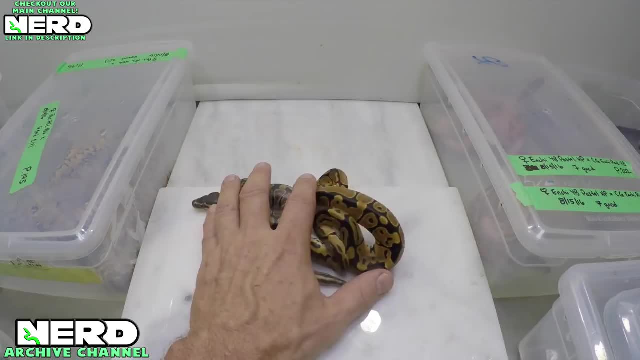 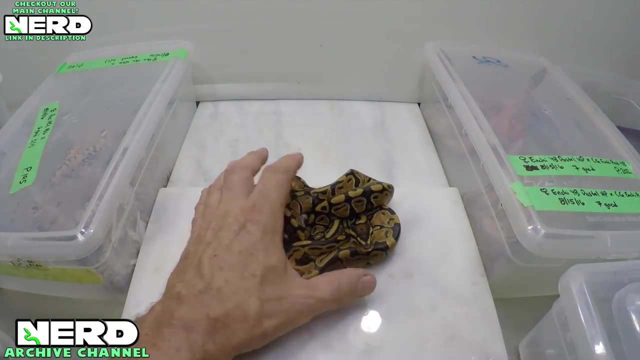 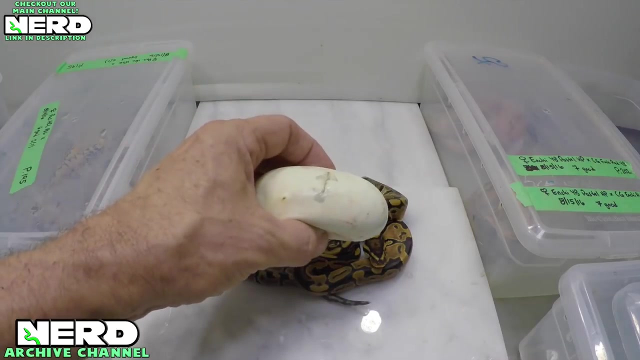 and I bred these together. what I would do, let's say, if we had four eggs, the probability per egg in this, from a het to a het from the previous clutch you'd have, each egg would have the probability of being 25%. the visual recessive. 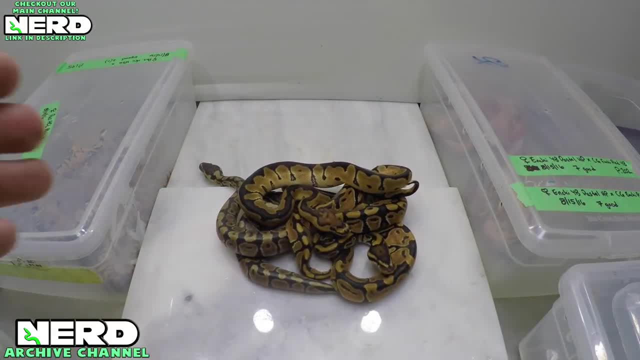 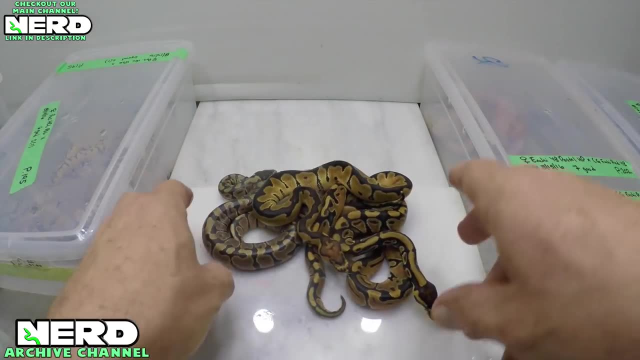 So in this case it's clown. So if I had four eggs, the theoretical probability would be 25% the visual heterozygous: 25% the visual heterozygous, 25% the visual heterozygous. 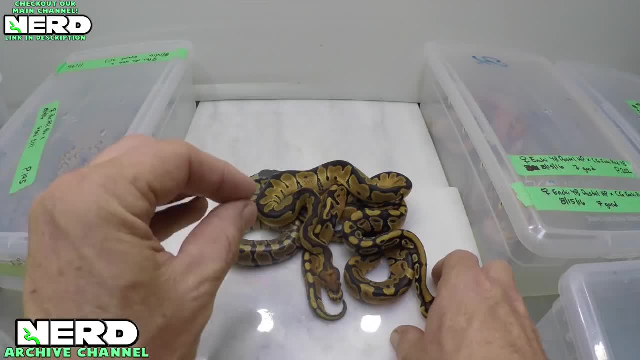 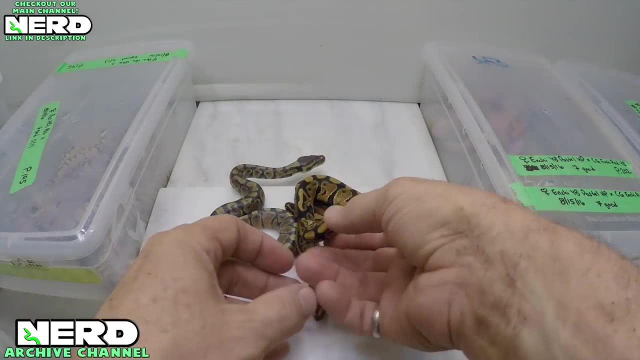 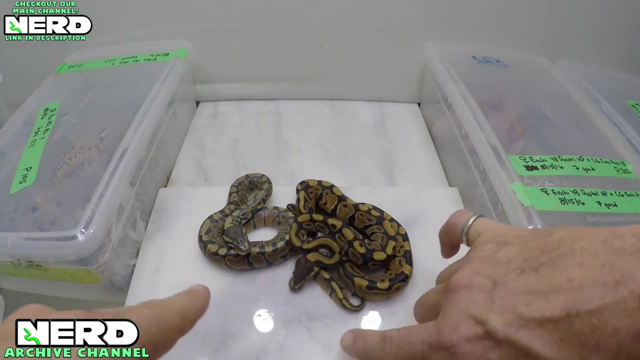 50% heterozygous, 25% normal. So if I remove the clown, the remaining babies, these are called probable hets, which means in theory two of the three are heterozygous gene carriers, but I cannot guarantee visually discern. 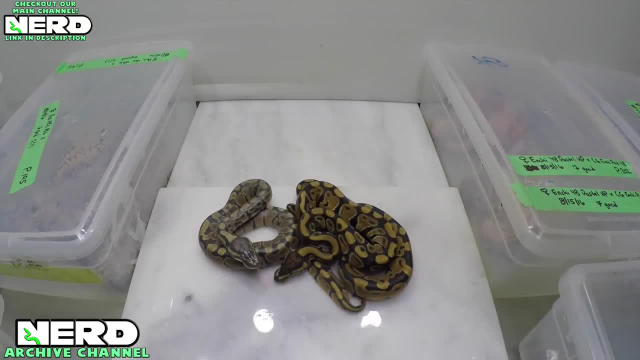 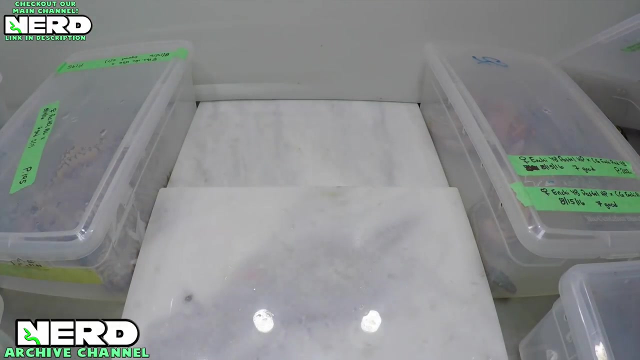 the difference between the two hets from the normal. So these are called 66% possible heterozygous for clown. That's a fact. this is all how it works. this is probability. So what happens if I now bred a clown to a het? 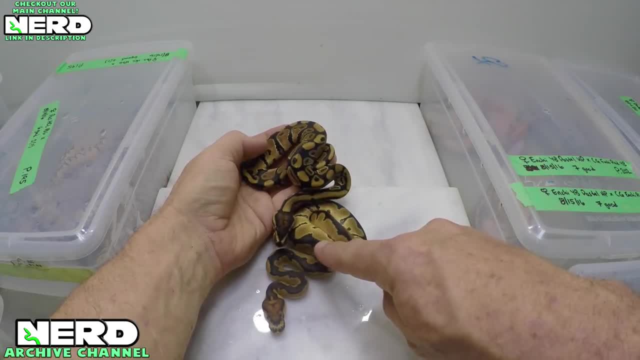 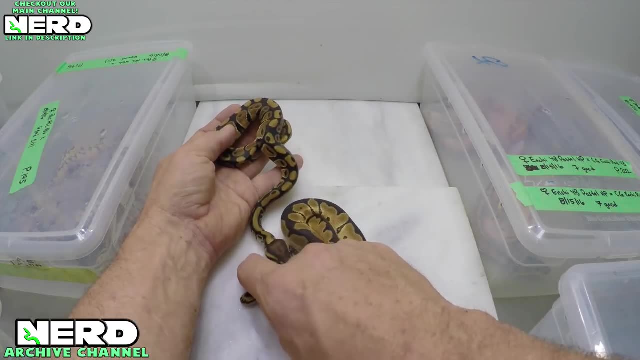 And if I raise these up, so this is a recessive clown. so basically, this is the homozygous expression of the gene, So it's the full expression of the gene. when I breed two hets together, I can make the homozygous full expression of the clown. 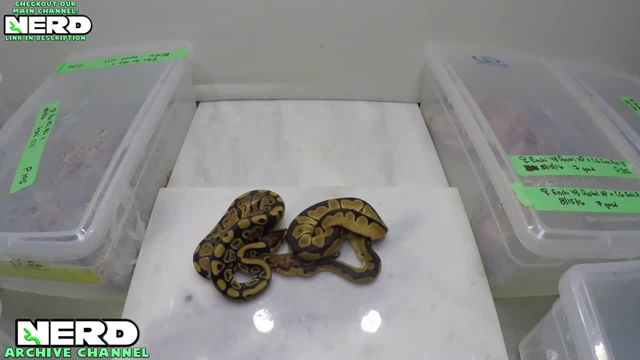 So if I breed two hets together I can make the homozygous full expression of the clown. So if I breed a het to a visual and I did four eggs and I looked at probability, each egg would give me a 50% chance. 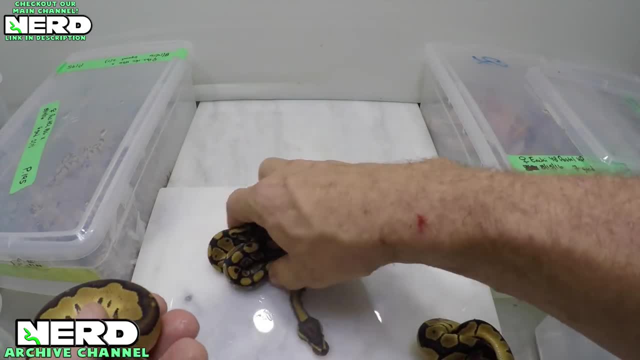 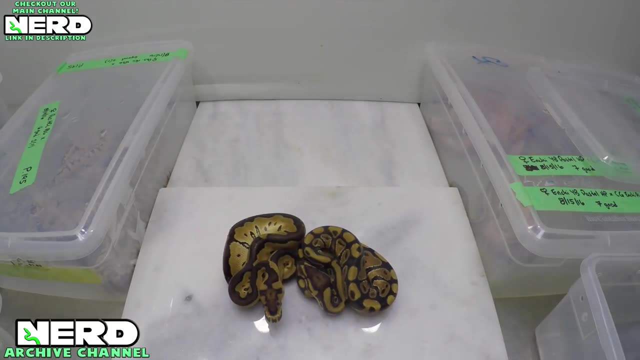 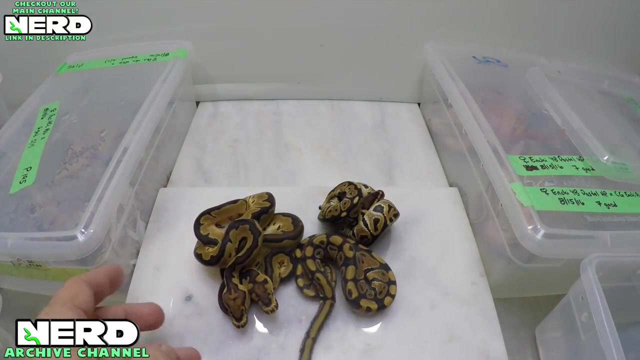 of being a clown And it'd also have a 50% chance of being a heterozygous. But what would happen was I would literally, if I had four eggs and I hit my probability, I could have two clowns. 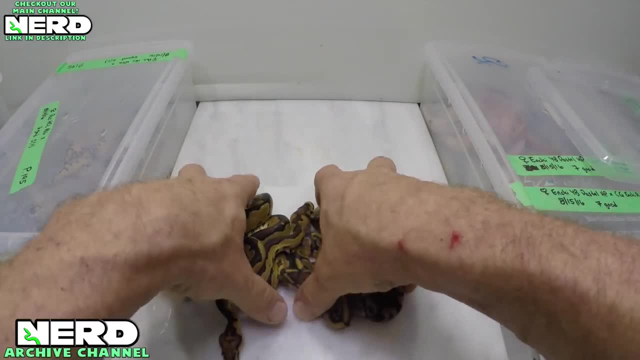 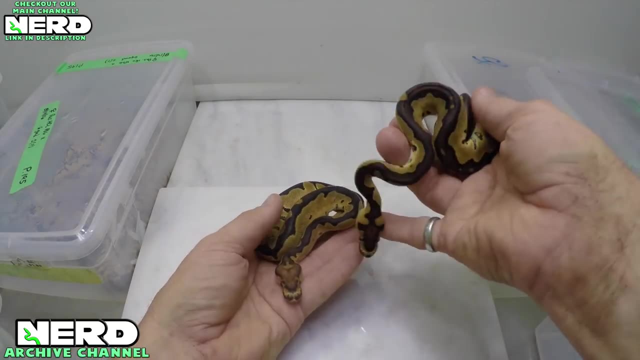 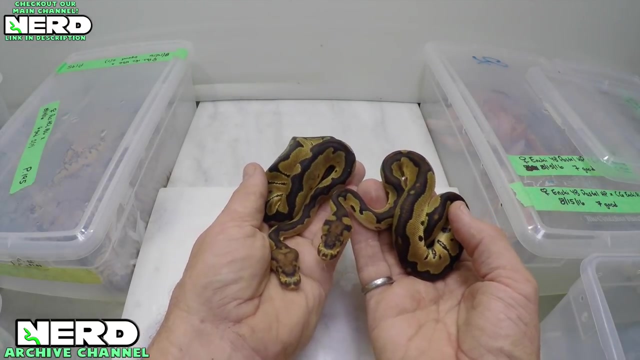 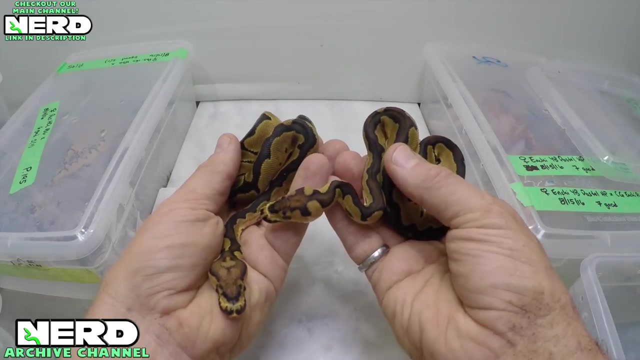 and two heterozygous. So if I take and breed a clown to clown both recessive genes together, all resulting babies will be the homozygous clown expression. This behaves the same with albinism, same with piebald, it's all the same.